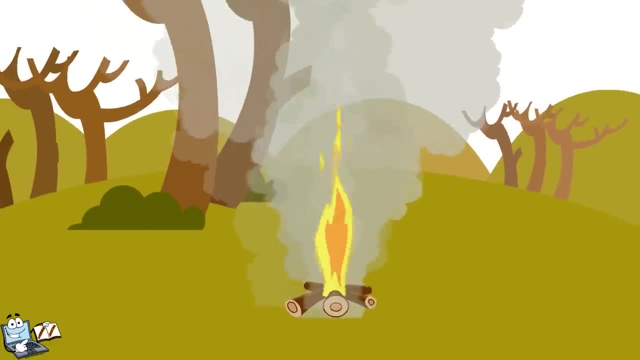 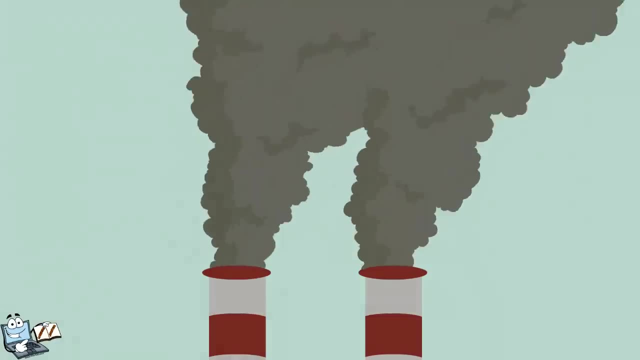 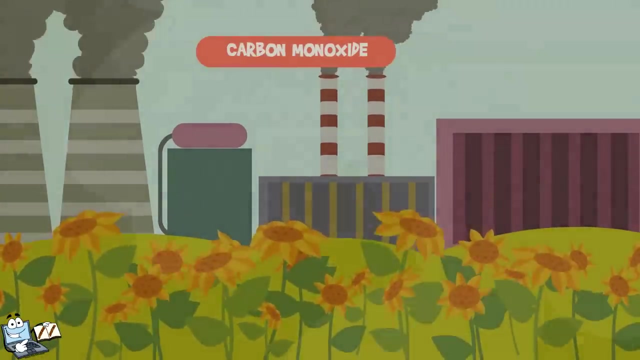 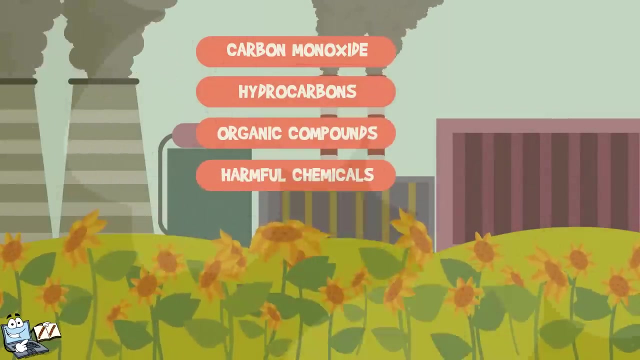 The smoke released from burning fossil fuel is also a major cause of air pollution. It includes oil, coal and natural gas. A large number of industries are also causing the release of industrial smoke and dangerous gases like carbon monoxide, hydrocarbons, organic compounds, harmful chemicals and more from the mills and factories to the environment. 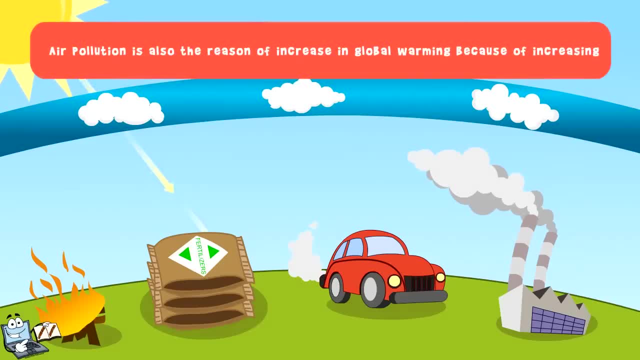 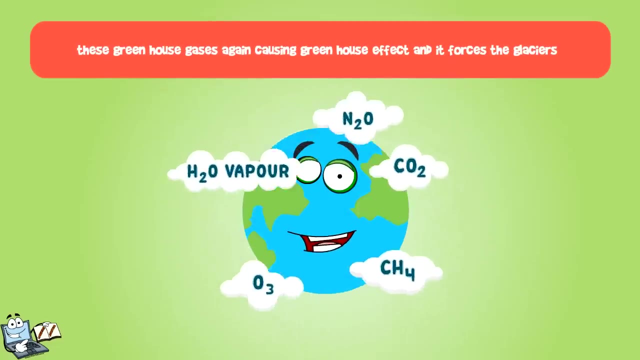 Air pollution is also the reason of increases in global warming because of increasing atmospheric temperature due to the vast increasing level of greenhouse gases. These greenhouse gases again cause the greenhouse effect. It forces the glaciers to melt, sea levels to increase and our climate to change. 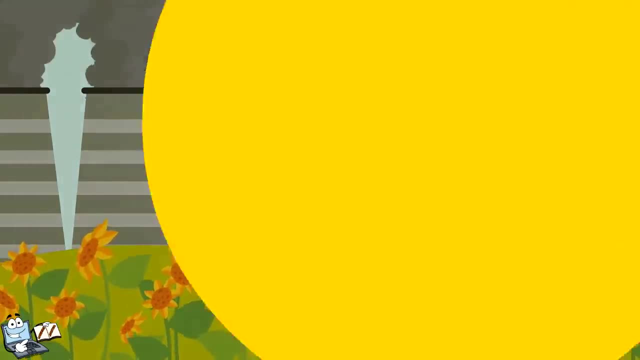 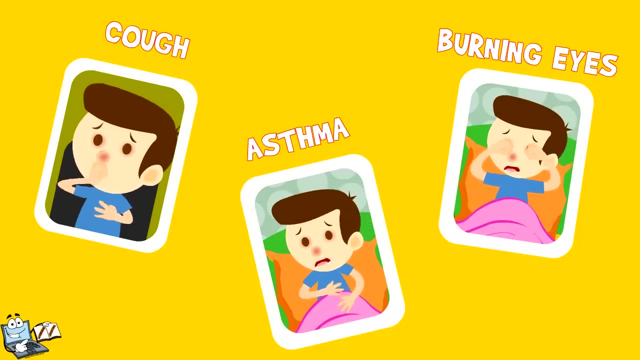 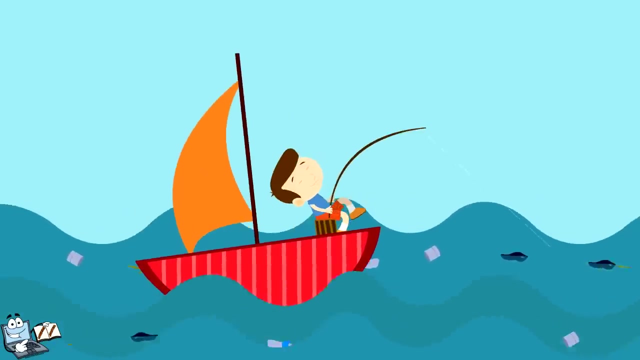 Air pollution is one of the major causes of coughs, asthma, burning eyes and also some lethal diseases like cancer, bronchitis, heart attacks, kidney diseases. Air pollution is one of the major causes of coughs, asthma, burning eyes and also some lethal diseases like cancer, bronchitis, heart attacks, kidney diseases. 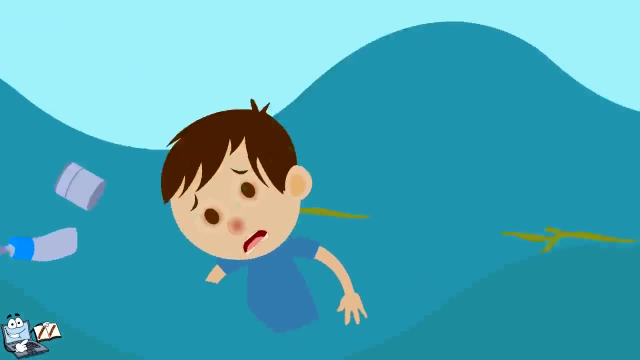 Air pollution is one of the major causes of coughs, asthma, burning eyes and also some lethal diseases like cancer, bronchitis, heart attacks, kidney diseases. Now we will learn about water pollution. It is the worst and most dangerous form of pollution. 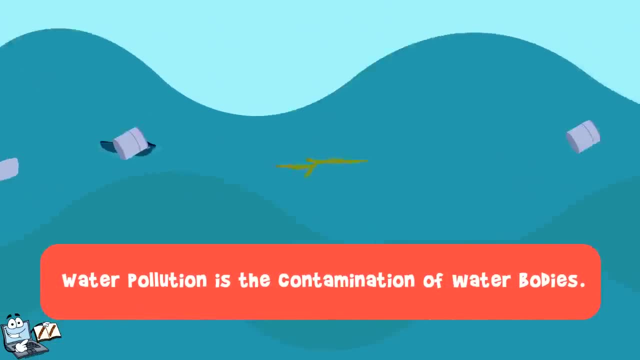 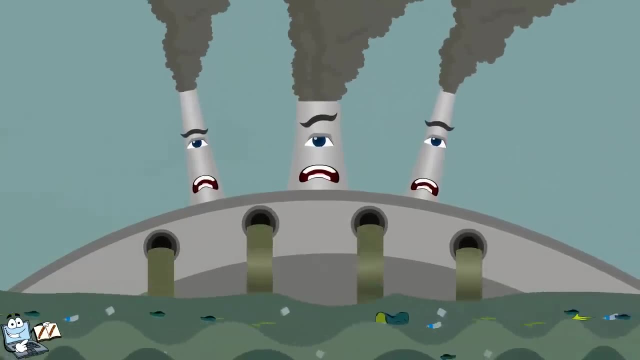 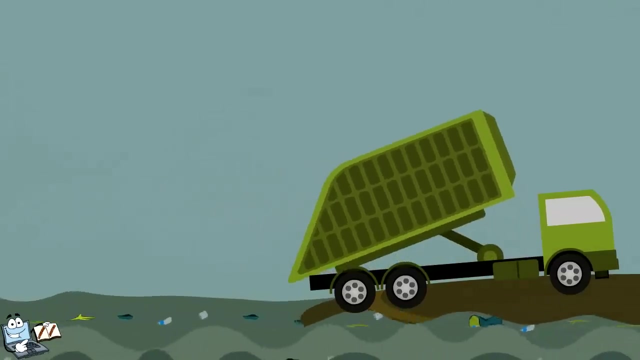 Water pollution is the contamination of water bodies. Water pollution happens when dirty particles, substances or chemicals that make water contaminated are discharged indirectly or directly into the water. Water pollution happens when dirty particles, substances or chemicals that make water contaminated are discharged indirectly or directly into the water. 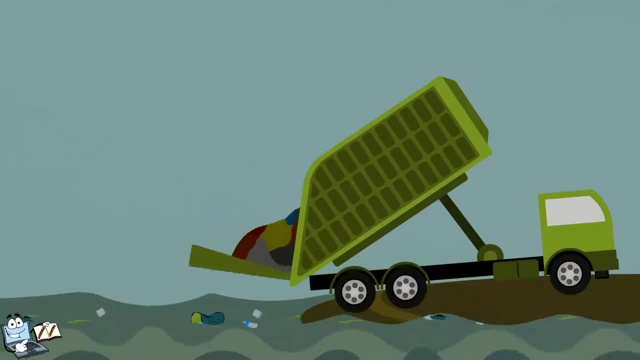 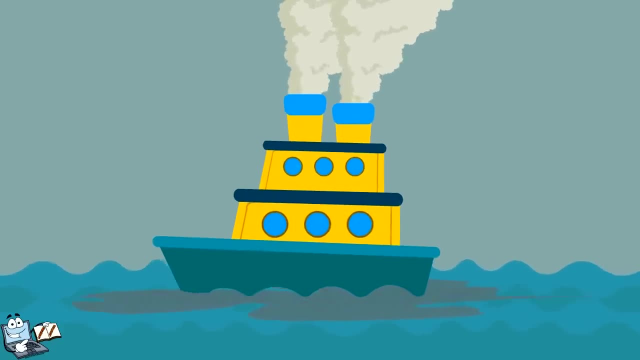 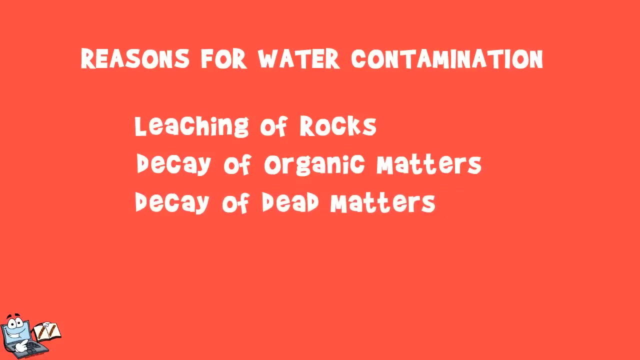 Pollutants get into water, mainly by human causes or human factors. Oil is also a big pollutant for polluting the water. Leaked oil from the ship or other modes flows to the sea or ocean and affects the whole water. There are some other reasons too for water contamination, like leaching of rocks, decay of organic matter, decay of dead matter, silting oil, erosion and more. 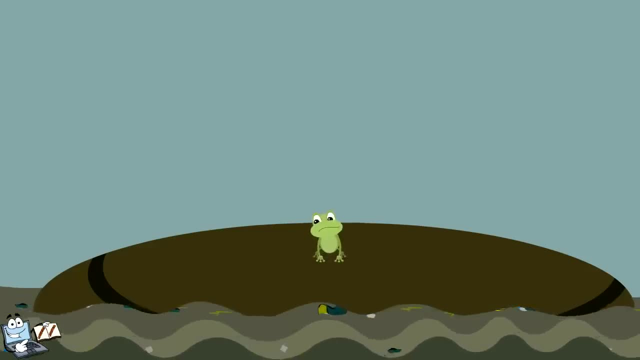 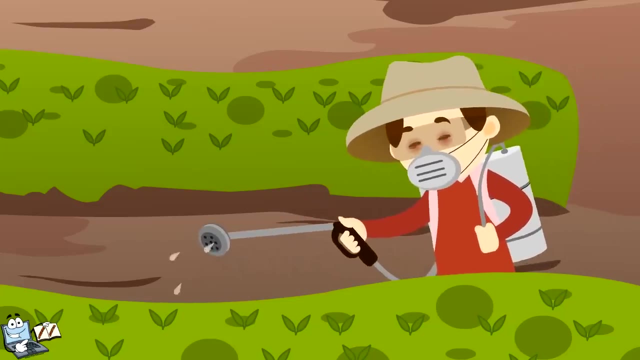 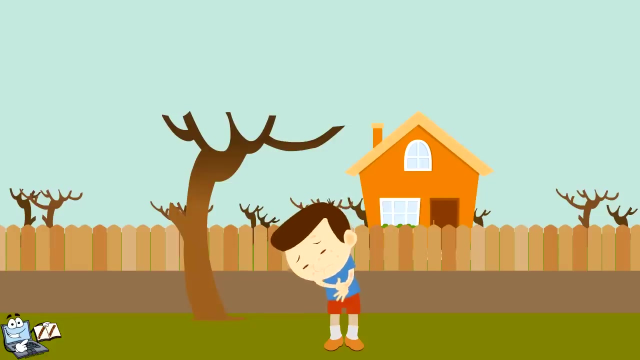 Water pollution also affects the population and entire functioning ecosystems that live in the waters. Some substances used by farmers to kill pests or weeds could seep into the ground and make the groundwater unfit to drink. Dirty water may cause skin disease, anorexia, dysentery, amoebiasis and more.